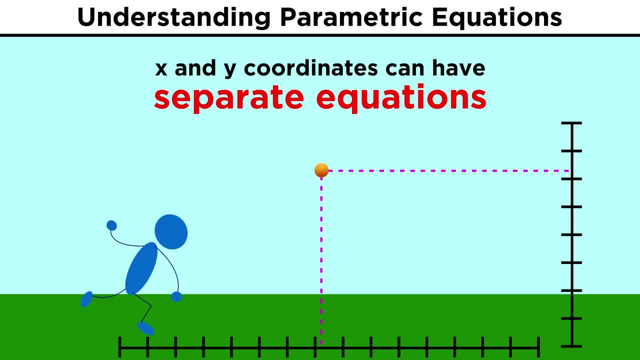 that models the X coordinate of the ball with respect to time and an equation that models the Y coordinate of the ball with respect to time, as they do indeed depend on the parameter of time differently and we may sometimes want to ask a question about one of these. 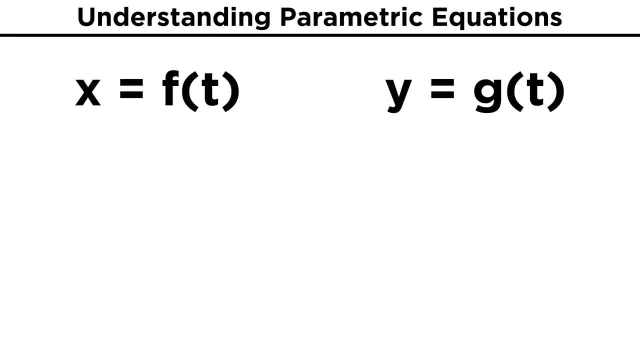 values and not the other. So we can say that in general sets of parametric equations come in the form of X equals F and Y equals G, two separate functions, but they depend on the same parameter. Then to graph the plane curve that results, we can just plug in some values of t and see. 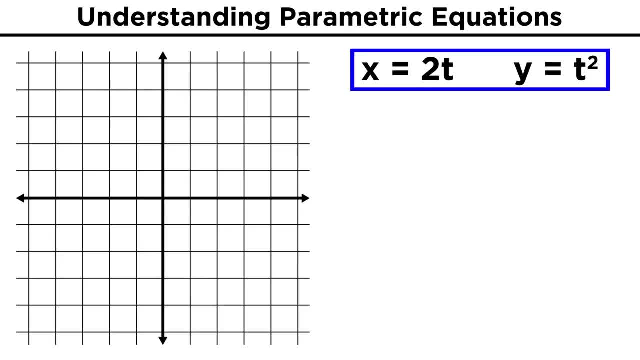 what we get. For example, let's look at the parametric equations: x equals two t and y equals t squared. Let's make a little table, pick some t values and then find the corresponding x and y values. Once we have all of these, we essentially have a set of x and y coordinates, so we can. 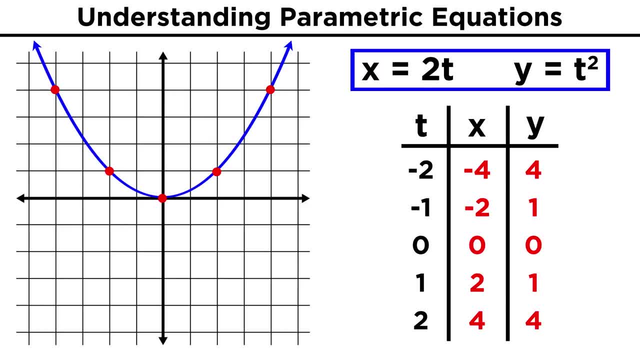 now plot all of these points, connect them and we see that we get a parabola. We can quite easily get the equation for this parabola by doing something called eliminating the variable. This is where we solve for t in one of the equations and plug it into the other. 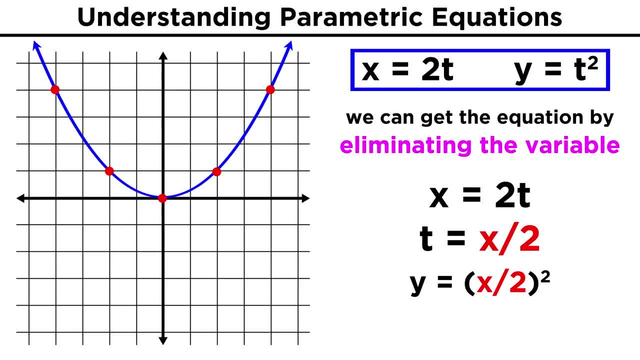 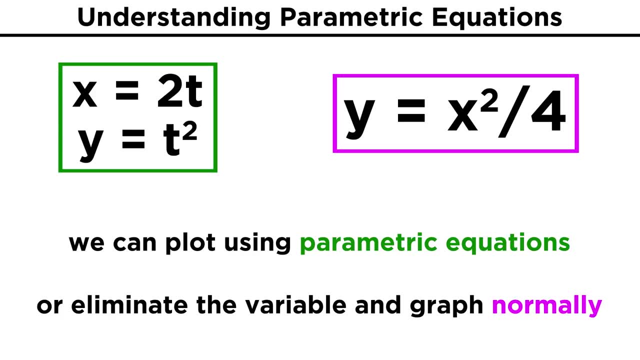 Using this one, t must be equal to x over two. so let's plug x over two into the other equation And we get y equals x squared over four, or one fourth x squared, Depending on the situation. it can be easier to plot points using the parametric equations. 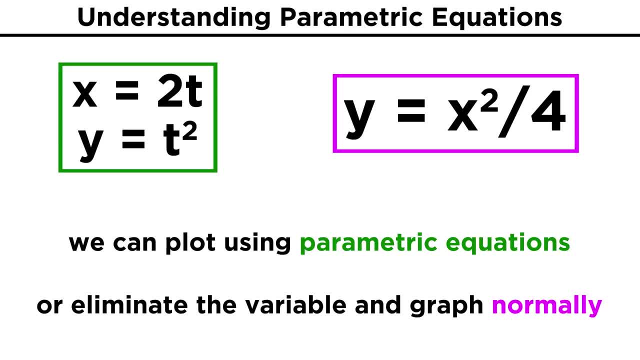 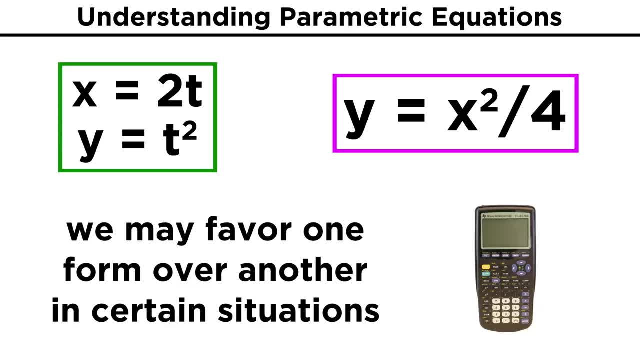 or to find a way to eliminate the parameter and just graph it. normally There are different situations that would favor one approach over the other, For example, if, using a graphing calculator, it can be easier to enter the equation of something like an ellipse in parametric form. 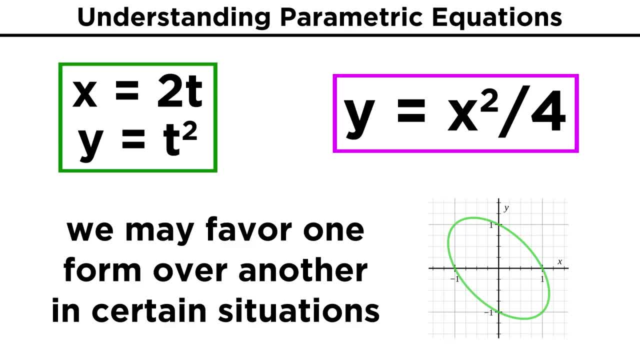 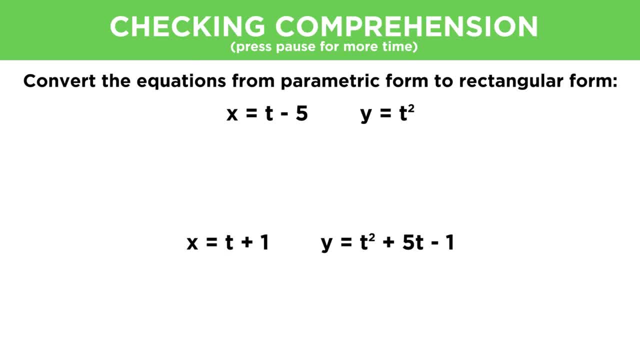